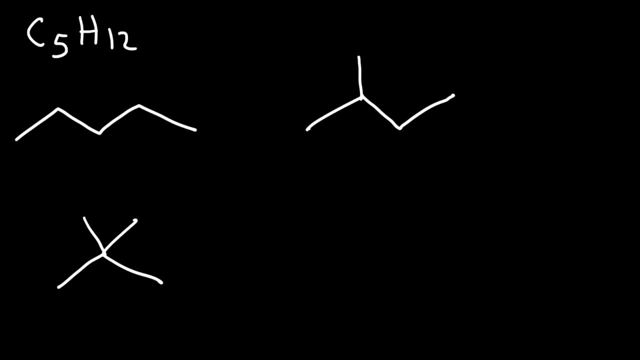 groups on carbon 2.. And so these are the three constitutional isomers of pentane. Now, what about for hexane? How many constitutional isomers can we draw for this molecule, C6H14?? So the first one. let's start with a. 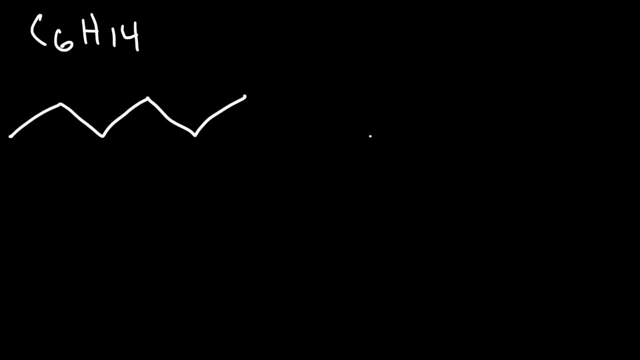 straight-chain alkane. That's one. Now let's go down to five carbons and let's add a methyl group on carbon 2. We could also put a methyl group on carbon 3.. Now we can't put a methyl group on carbon 4. 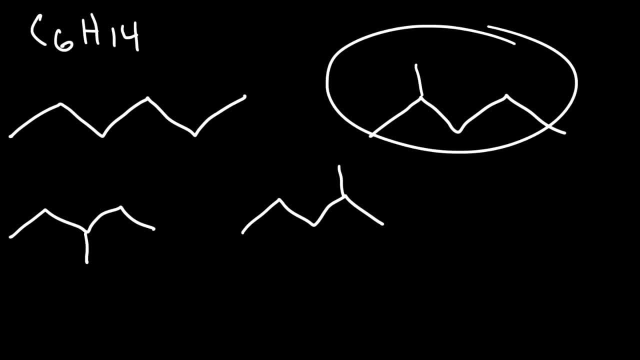 because these two are identical. They're not constitutional isomers. In fact, if you try to name it, they will have the same name. So this would be called 2-methyl pentane, And then for the other molecule you have to count in the other. 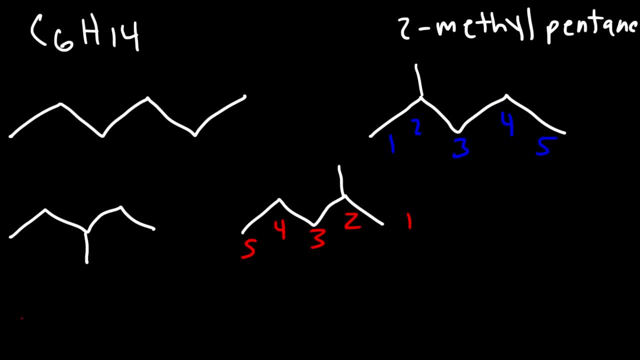 direction going from right to left. So, as you can see, it has the same name: 2-methyl pentane. Now, if we name the structure on the left, notice that this is called 3-methyl pentane, And so it's important to understand that constitutional isomers. 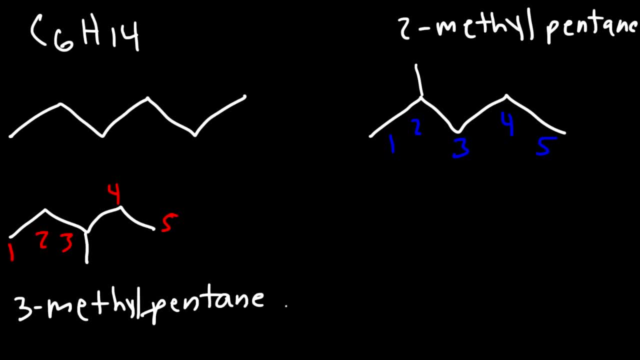 they have the same molecular formula, but they're connected differently and also have different names. The nomenclature cannot be the same. So let's see what other isomers we can draw. So let's go down to four carbons and we need to put two methyl groups So we can. 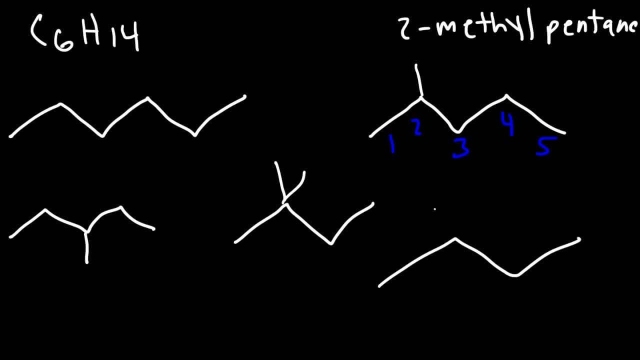 place both methyl groups on carbon 2, or we can spread it out: Put in one methyl group on carbon 2 and the other in carbon 3.. So for hexane I got five constitutional isomers. Now let's see how many we can draw for heptane: C7H16. 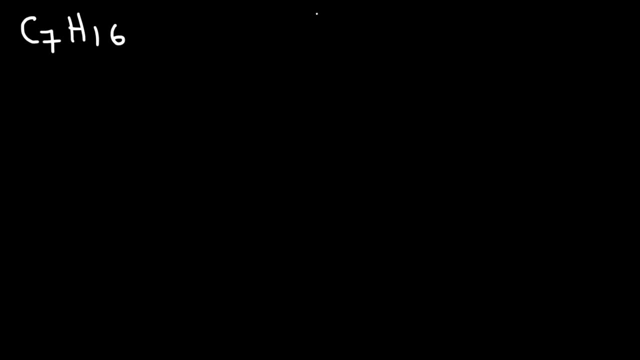 Feel free to pause the video if you want to try it. So first we can start with seven carbons in a straight chain, So that's a total of seven. Then we can go down to six carbons. We could put a methyl group on carbon 2, or we could put 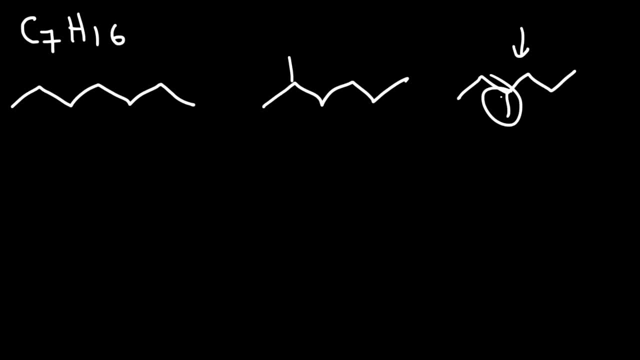 one on carbon 3.. If we place one here, it will be the same as putting it on carbon 3, or if we place it here, it's the same as putting it on carbon 2 from the left. Just keep that in mind. So now let's go down to five carbons, and so we need to. 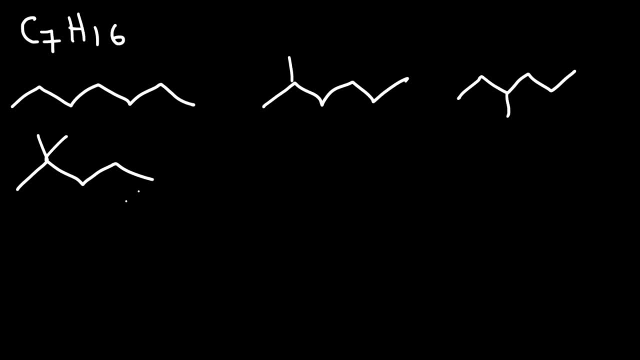 add two methyl groups. We can add both methyl groups on carbon 2.. Or we could add two methyl groups on carbon 3.. Or we can place one methyl group on carbon 2 and one on 3.. Or we could place one on 2 and one on 4.. So far, 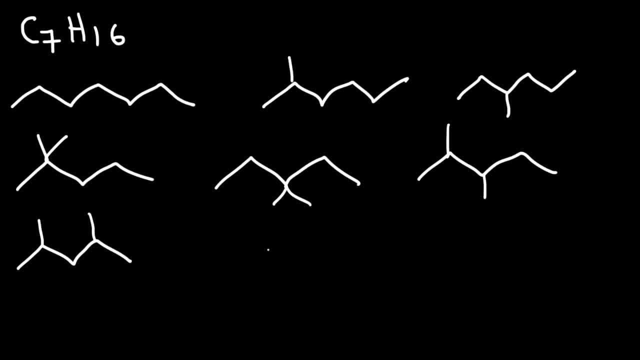 we have seven constitutional isomers. Now let's go down to four carbons. In this case we need to add three other carbons, So we can place two methyl groups on carbon 2 and one on 3.. And I've believe that's it for the four carbon chain. But you know what, If we go back to 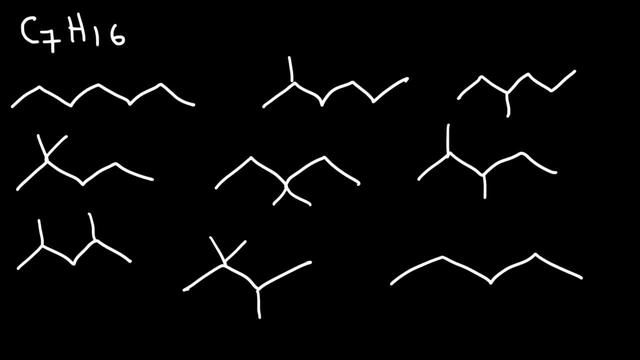 the five carbon chain. what we could do is we can place an ethyl group on carbon three And that's going to give us a completely different structure than anything we have seen. So for the five carbon chains, For this one, this is 2,2-dimethylpentane, This one is 3,3-dimethylpentane. 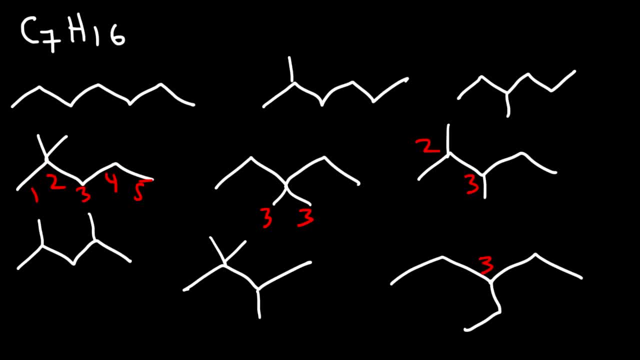 This 2,3-dimethylpentane, and this is 3-ethylpentane, So that's completely different from the others. And so we have nine constitutional isomers for heptane. Now let's move on to the next example, which is going to be octane. So for 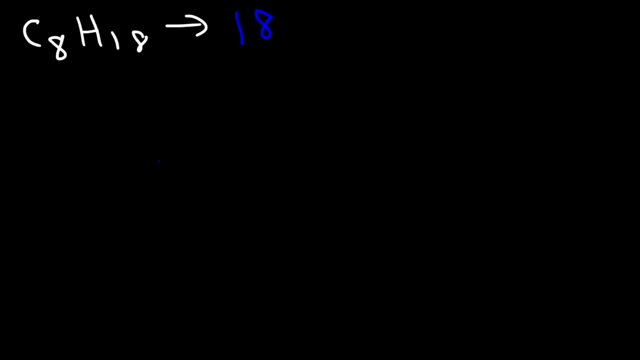 octane. there's a total of 18 constitutional isomers, So what I want you to do is pause the video and try to draw as many isomers as you can come up with. So let's start with an 8-carbon chain. So that's simply octane. Now let's go down. 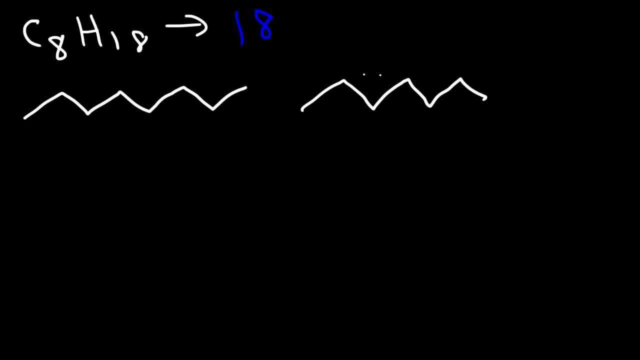 to 7, and we could put a methyl on carbon 2, or we could put a methyl on carbon 3, or we could put a methyl on carbon 4.. Now let's go down to a 6-carbon chain, So we can either place. 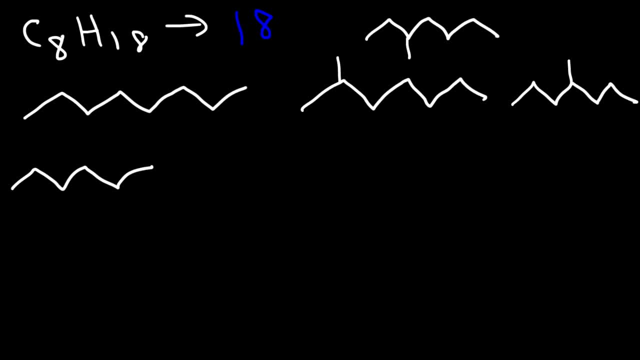 two methyl groups or an ethyl group, based on the last problem. So let's start with two methyl groups on the same carbon, So we can place it on carbon 2 or carbon 3.. Now we can place two methyl groups on different carbon atoms. Let's 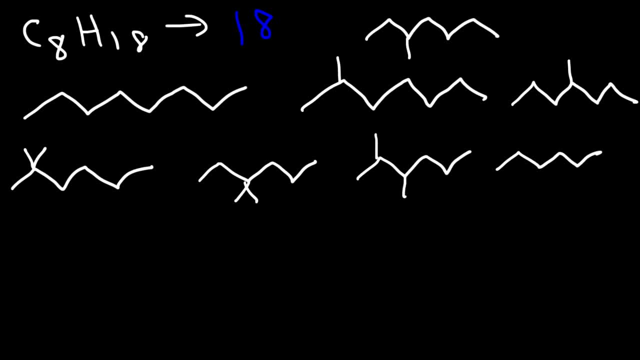 say carbon 2 and 3, 2 and 4 or 2 and 5.. We can also place a methyl group on carbon 3 and on carbon 4, because that will be different as well. Now let's talk about adding the ethyl group. Where can we add the ethyl group? 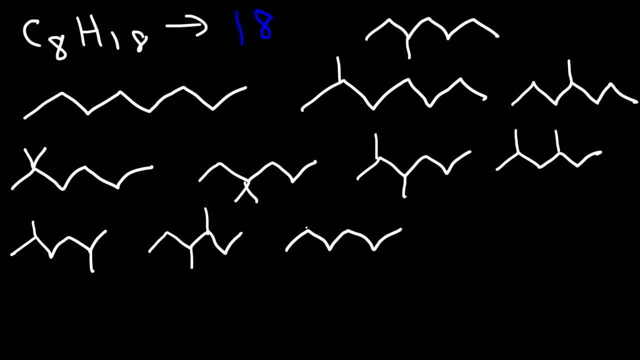 and where should we not add it? We cannot add it on carbon 2, because the longest chain won't be 6 carbons. it's going to be 7 carbons, And so what we're going to have is 3-methyl-heptane. 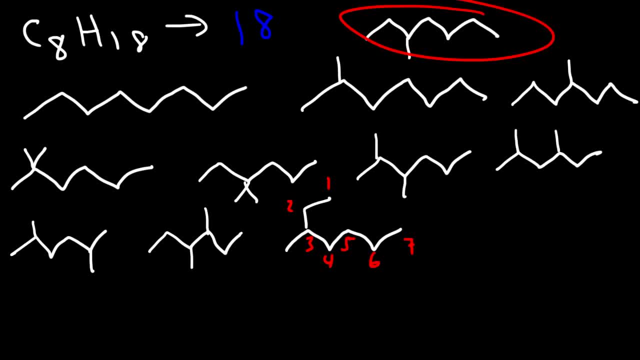 Which is the same as this one. So when adding the ethyl group, we have to add it to the third carbon or more, in order that the plant chain will not have more than 6 carbons. So we can add it on carbon 3 or on carbon 4, which becomes 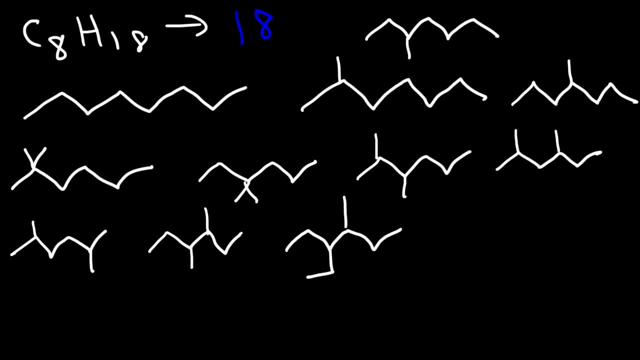 carbon 3 if you count it in the other direction. So there's only one location where we can add the ethyl group for a 6-carbon chain. Now let's go down to a 5-carbon chain So we can add 3-methyl groups, or we can do an ethyl and a methyl. 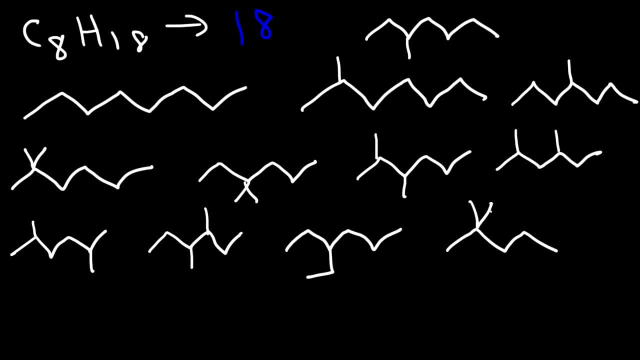 Let's start with 3-methyl groups. We can place 2 here and 1 here, Or we can place 2 on carbon 2 and 1 on carbon 4.. We could place 2 on carbon 3 and 1 on carbon 2.. 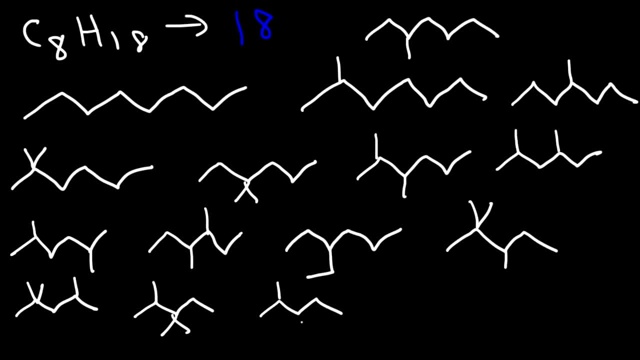 Or we can place 1 on carbon 2,, 3 and 4.. Now let's talk about the ethyl group that we can add. So we can add an ethyl group on carbon 3 and then we can add a methyl on carbon 2.. Or we can add the. 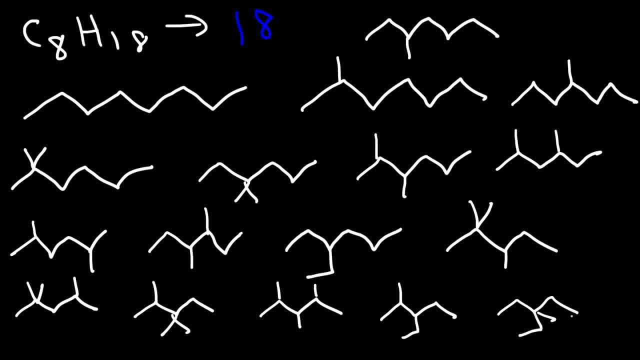 ethyl group on carbon 3 and the methyl on carbon 3.. So let's count how much we have so far. So this is 1,, 2,, 3,, 4,, 5,, 6,, 7,, 8,, 9,, 10,, 11,, 12,. 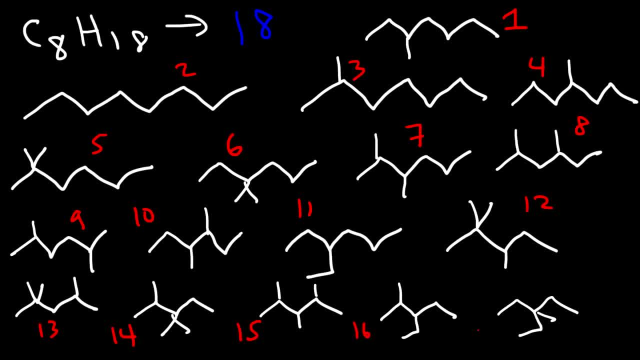 13,, 14,, 15,, 16,, 17.. So far we have 17 constitutional isomers. We need one more. So what do you think the last one could be? Well, we can't go down to 4 carbons. Maybe we could go down to 4 carbons If. 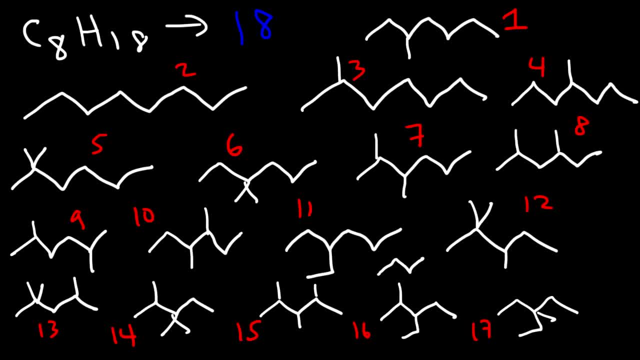 we go down to 4 carbons, we have to add 4 more carbons to get 8 carbons. So we could put 2 on carbon 2 and we could also put 2 on carbon 3.. So that that's 18.. 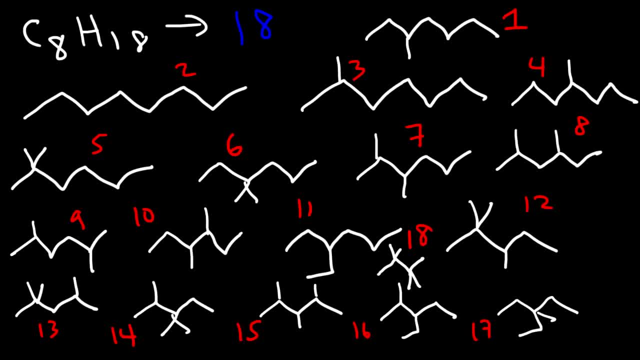 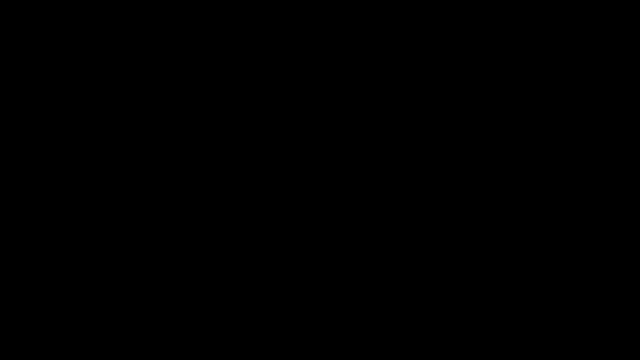 So these are the 18 constitutional isomers of octane. Now what about this one, C2H6O? How many different constitutional isomers can we draw? So we can draw an ether. This is dimethyl ether. It has 2 carbons, 6. 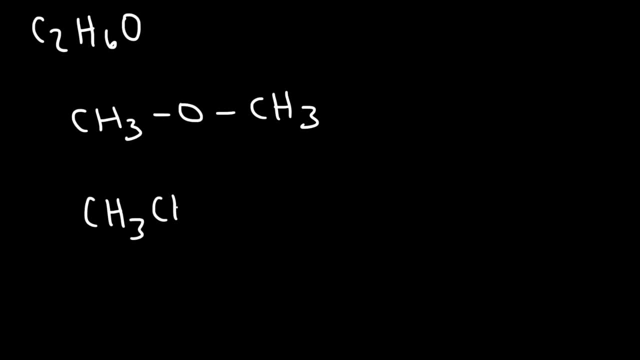 hydrogens and an oxygen, Or we can represent it as an alcohol. Now, what about this one, C4H8. We did C4H10,, which was an alkane. It had the formula CnH2, 2n plus 2.. This one has the formula CnH2n. When you see, 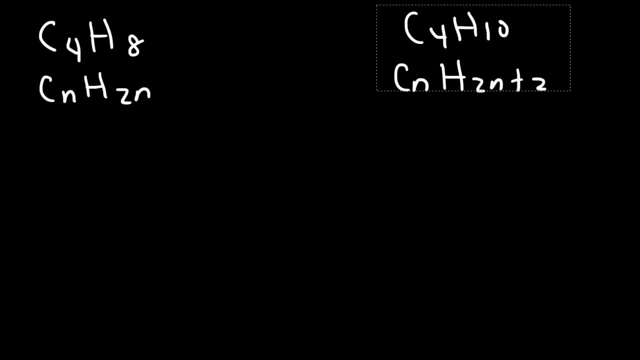 that it's either an alkane with one double bond or it's a ring. So for C4H10, we can draw this isomer. So this isor isoisomer is for voucher, because it'sале�로ge. But all of these 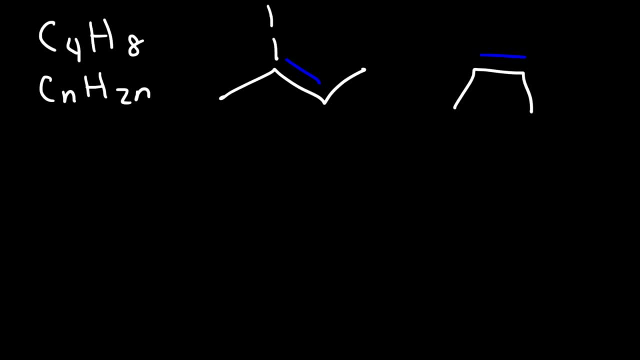 are isomers for voucher, So we are just trying to see if there's any chance that there's anything that gets sawed off from the end of the serum. Now, to see how they react, we can draw 1 diethyl addiotyloide, or to see if we can. 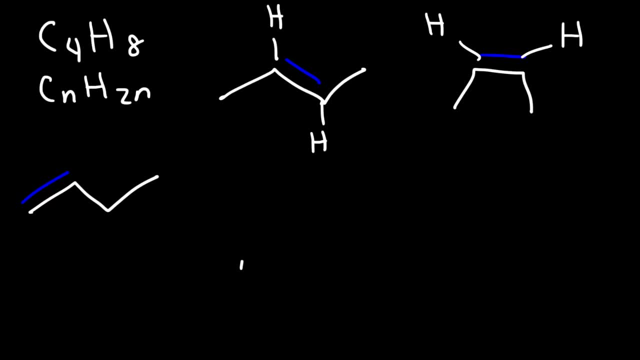 see what they say. We can also draw all the different ec cav. These are cis trans and electrostimula bikini. We can also draw cis trans to btine. We can also butane, cyclobutane. Notice that each carbon has two hydrogens. We can draw a. 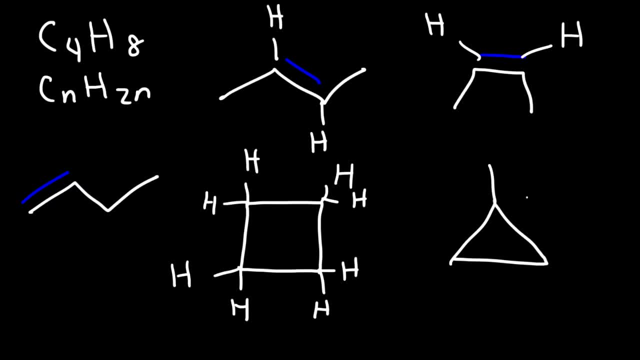 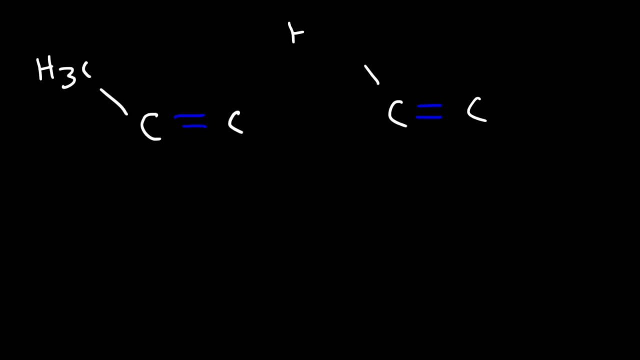 cyclopropane ring with the methyl group, And so those are some different ways in which we can draw a structure with this formula C4H8.. Now let's talk about cis and trans-tubutene. The reason why they're not constitutional isomers is because they're